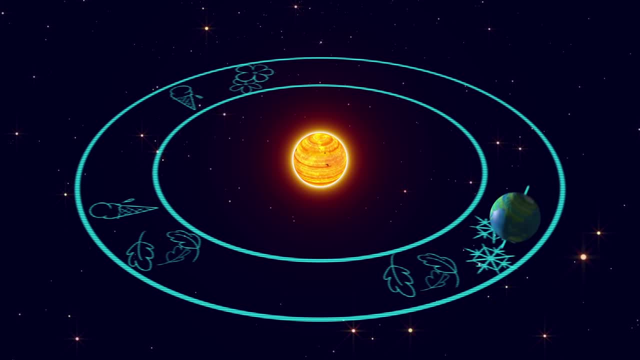 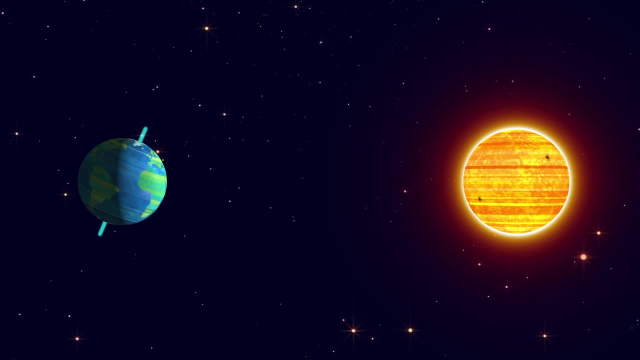 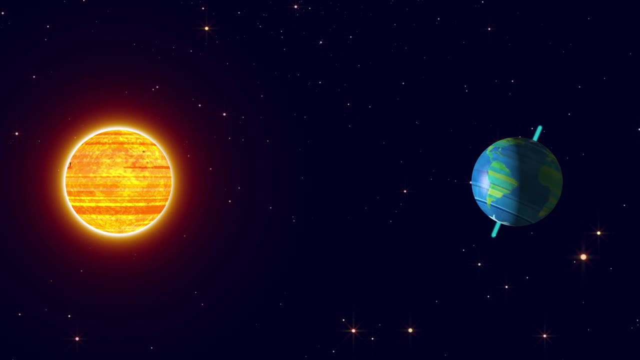 Because the axis remains tilted in the same direction while the Earth makes its annual orbit. there are long periods each year when the northern half of the planet remains tilted toward the sun while the southern half is tilted away, and vice versa. what we experience as summer and winter. 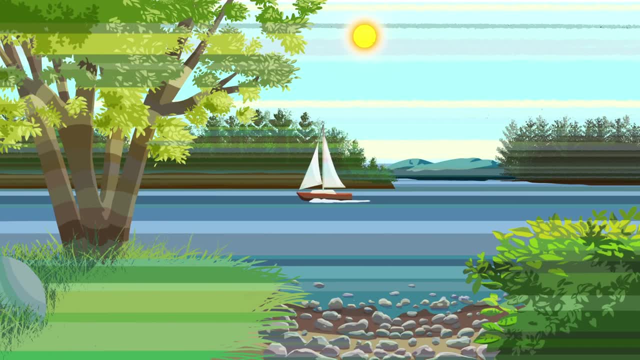 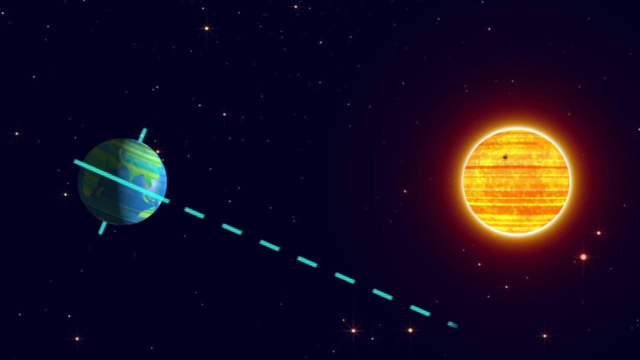 During summer, in a given hemisphere, the sun appears higher in the sky, making the days longer and warmer Once a year. the sun's declination: the angle between the equator and the position on the Earth where the sun appears directly overhead. 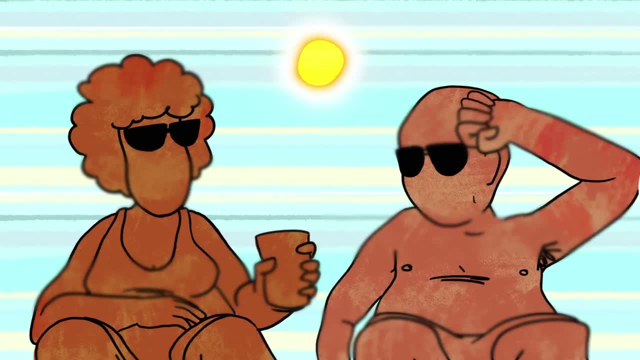 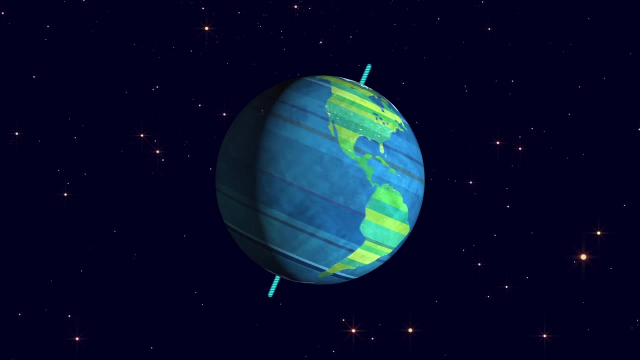 reaches its maximum. This day is known as the summer solstice, the longest day of the year and the one day where the sun appears highest in the sky. So the Earth's axial tilt partially explains why the sun changes positions in the sky. 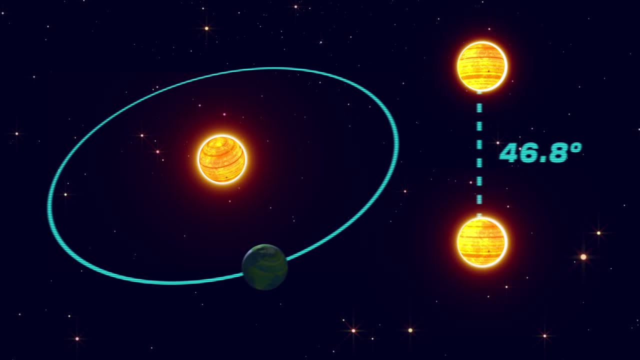 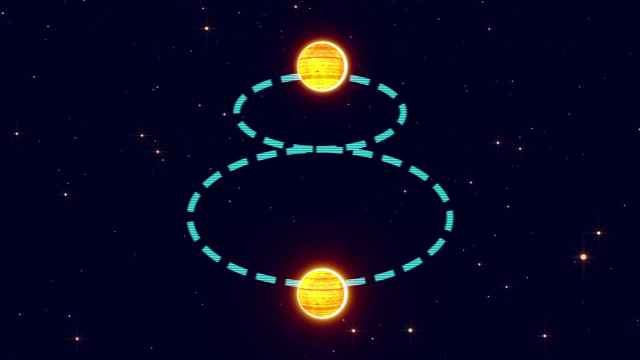 and the analemma's length represents the full 46.8 degrees of the sun's declination throughout the year. But why is it a figure eight and not just a straight line? This is due to another feature of the Earth's revolution. 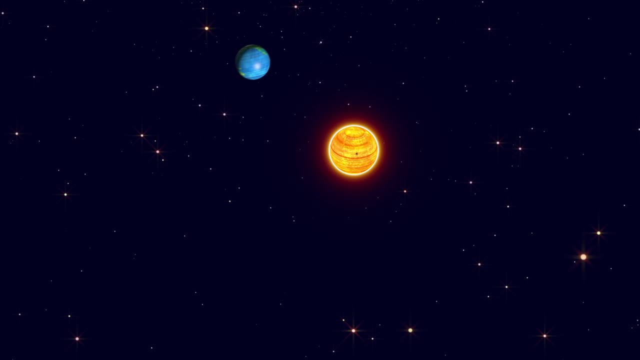 its orbital eccentricity. The Earth's orbit around the sun is an ellipse, with its distance to the sun changing at various points. The corresponding change in gravitational force causes the Earth to move fastest in January, when it reaches its closest point to the sun. 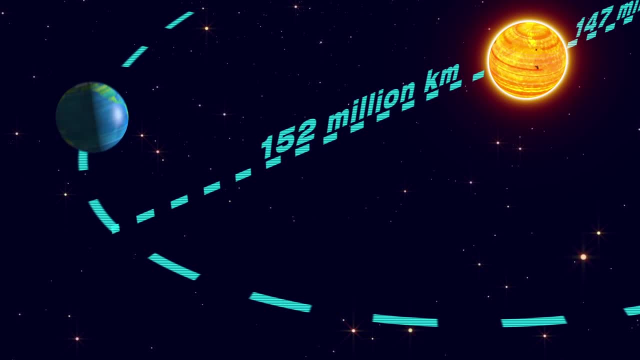 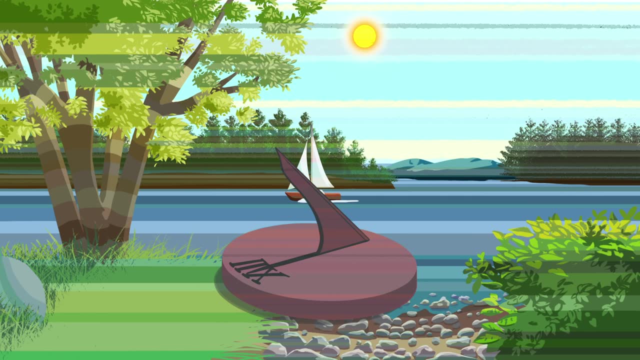 the perihelion, and the slowest in July when it reaches its farthest point, the aphelion. The Earth's eccentricity means that solar noon, the time when the sun is highest in the sky, doesn't always occur at the same point in the day. 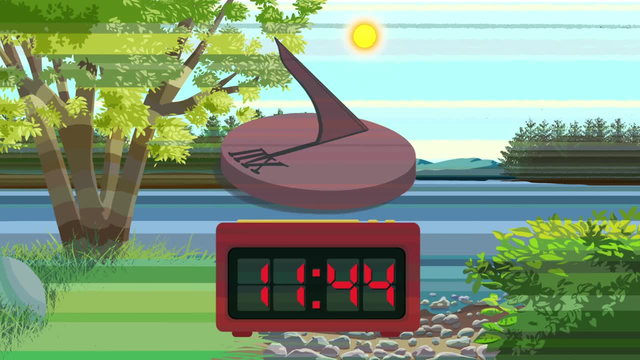 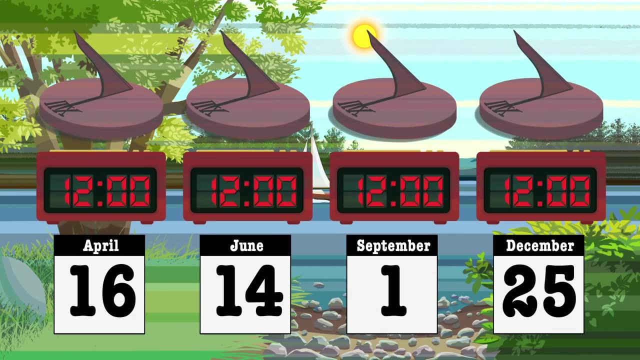 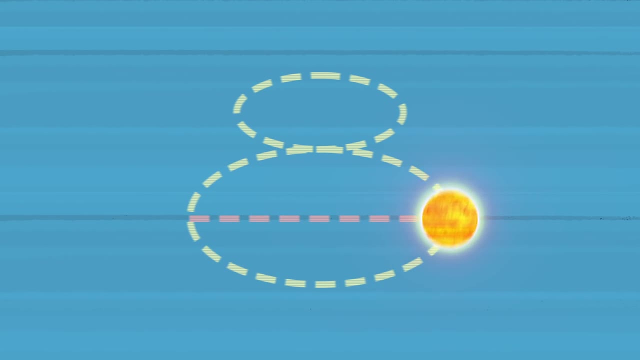 So a sundial may be as much as 16 minutes ahead or 14 minutes behind a regular clock. In fact, clock time and sun time only match four times a year. The analemma's width represents the extent of this deviation. 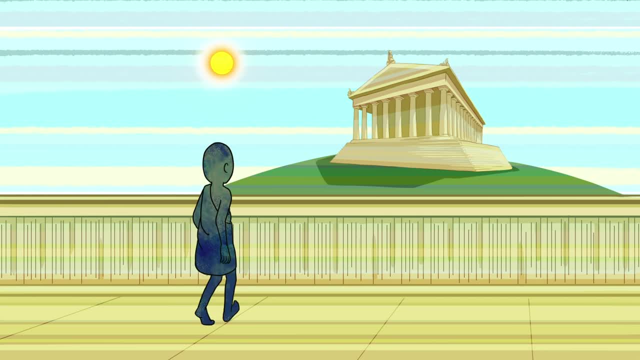 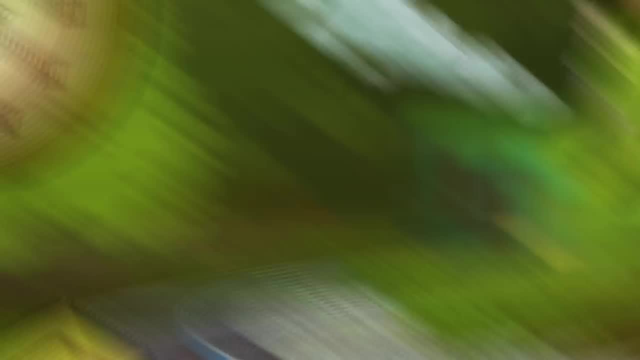 So how did people know the correct time? years ago, For most of human history going by, the sun's position was close enough, But during the modern era the difference between sundials and mechanical clocks became important, The equation of time introduced by Ptolemy.